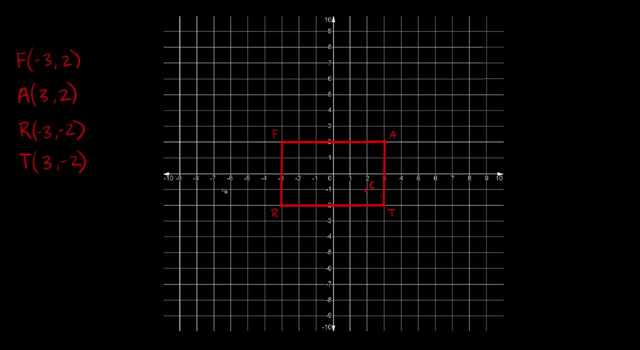 just, for example, to like right there, it would completely change what my dilation would look like, or the copied image, Okay. or sometimes you'll see this center of dilation or this dilation point on the outside somewhere, right, so it won't even be inside your shape anywhere, it'll just be floating on the outside. 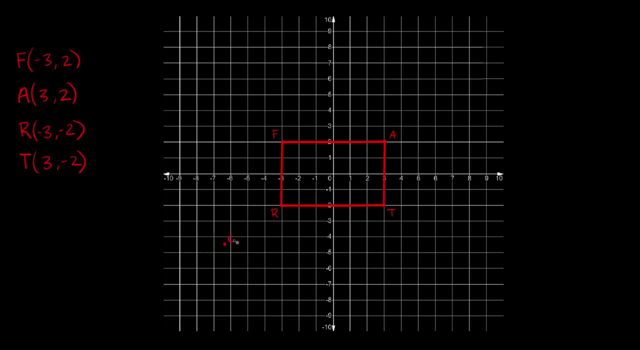 somewhere, and again that's going to change how you draw your dilation right. so, where this point is really really important- and the other thing that is really really important- is the scale factor. Okay, and that's denoted by the letter k, and the scale factor is just a number that tells you how. 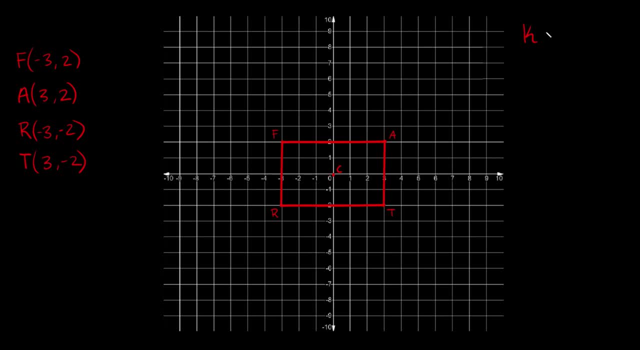 much you're going to increase or decrease the size of your shape. Okay, and whenever k is equal to one, your shape doesn't change, right? it's? it just stays exactly the same, right? but if k, for example, was equal to two, well then your shape would double in size. 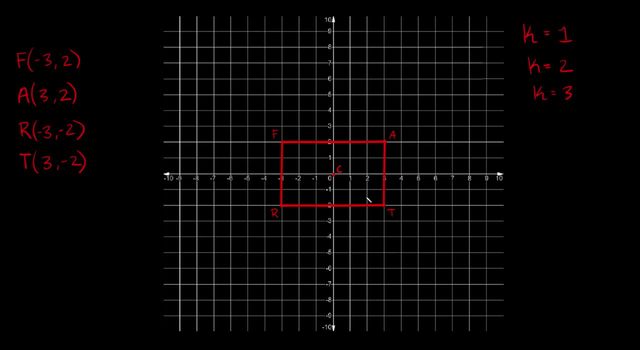 if k was equal to three, well then, your shape would triple in size. Okay. if k was equal to one half, well then your shape would be cut down or shrink by one half, okay, or by 50 percent, or you want to think about it. Okay. now a couple of things about k. K can't be equal to zero because 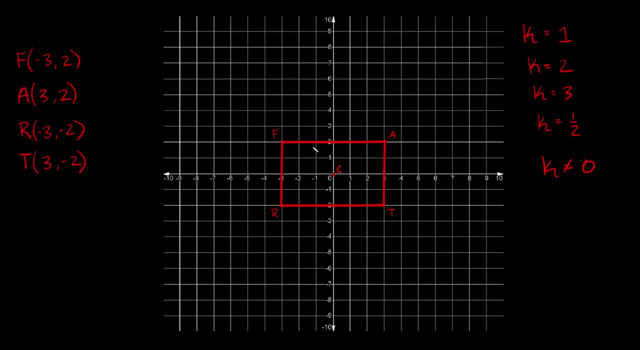 if it was ever equal to zero, you would have no shape. okay, this thing would just disappear. and also, k usually isn't negative. so in general, when k is between zero and one, okay. so when it's less than one, but it's more than zero, the shape shrinks. but if k is greater than one, 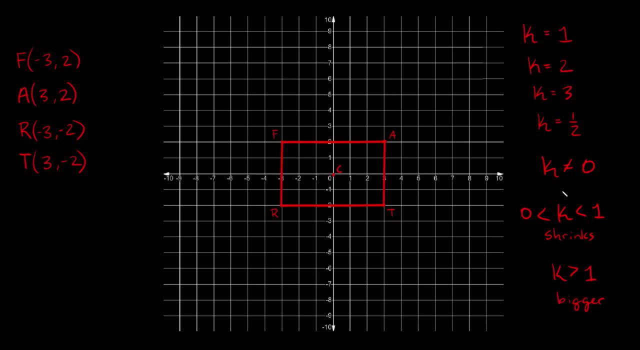 then your shape gets bigger. This is kind of the general rule that you'll see most places okay. so there's a little bit more to the scale factor that I want to cover, but that's kind of the gist of it. that's definitely enough to kind of get us started on an example. all right, So let's say we started. 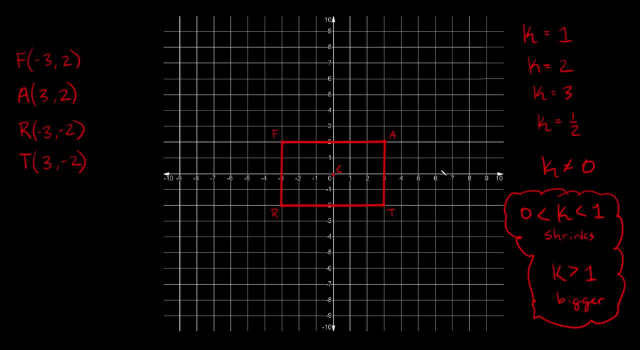 with this rectangle right here, right rectangle f a r t. now let's apply a scale factor of two. okay, so again, that means I want to double the size of my rectangle Over here, right? so how do we do that? well, there's basically two methods. so the first method: you can 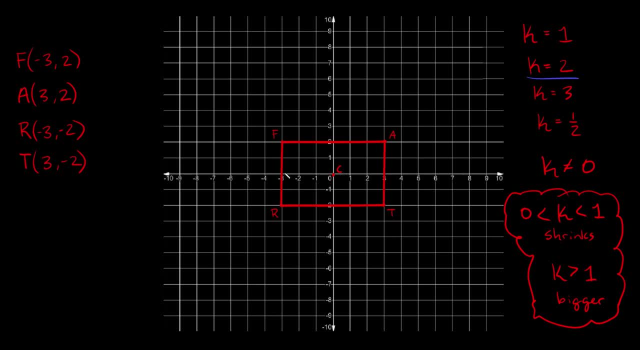 use is by just counting squares. Okay, so if we want to double the size of this big rectangle, we just have to figure out how far the center of dilation over here- all right- point c is to each of the points on our rectangle. okay, so how far is it from c to f, then from c to a? 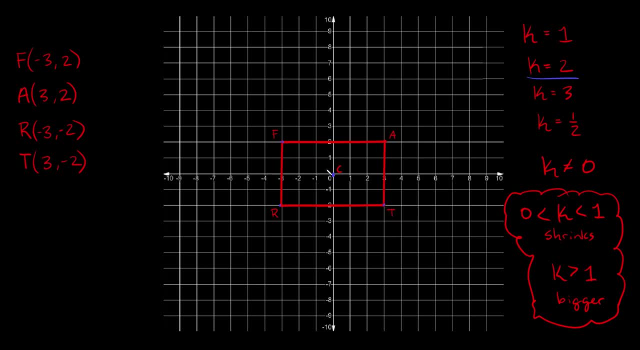 c to r and from c to t. okay, so, first of all, how Far Is C to F? Well, if you just counted spaces, we could go over 3 and up 2, right, We would go over 3 and then up 2.. So if we want to double that right, because we're applying the scale factor of 2,, 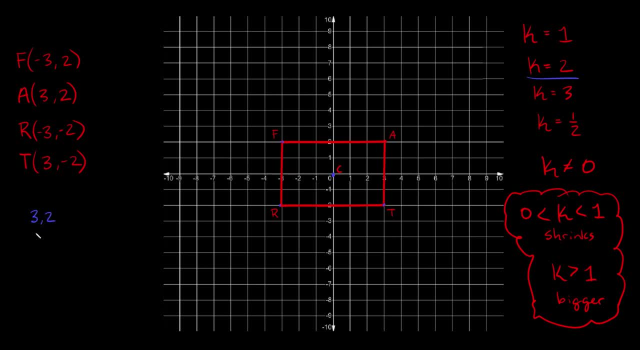 right, so we want to double it. we would just double these lengths. okay, So instead we would go over 6 and up 4,. okay, So instead of going just over 3,, we would go over 6, and then, instead of. 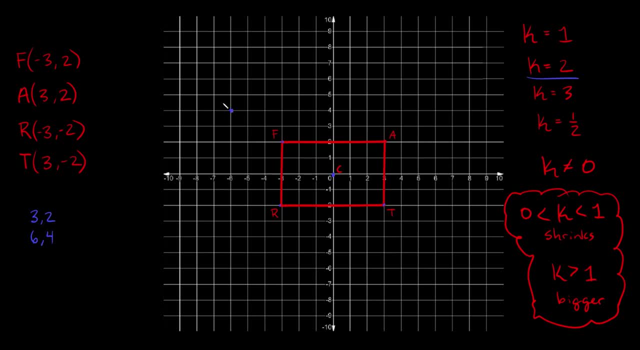 just going up 2,. we would go up 4, okay, So then this point right here would be F prime, and then we could do the same thing with the rest right. So from C to A, same thing. Right now we have to. 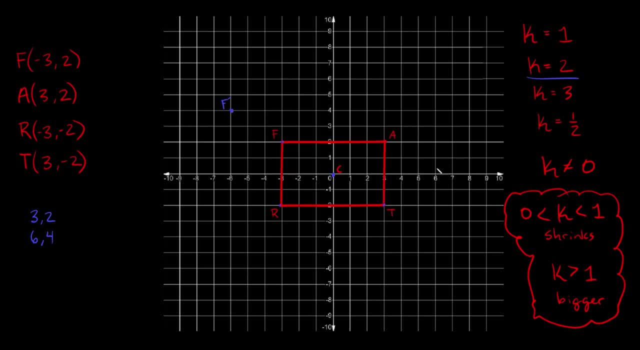 go over 3 and then up 2.. So to double that, we would go over 6 and then up 4, right? So then this point would be A prime and then I think you kind of see the pattern right. So from C to R: same. 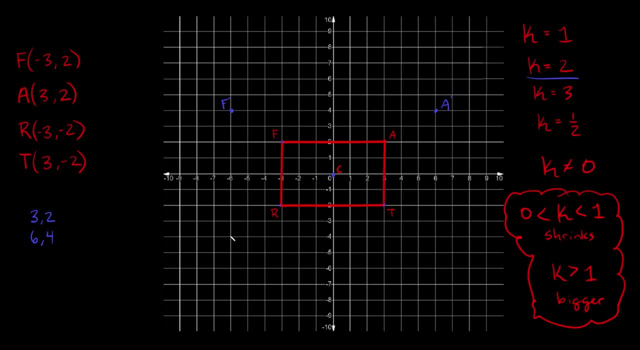 thing: over 3,, down 2.. So then we'd go over 6,, down 4, and then, from C to T, same thing: go over 6, and then down 4.. Okay, so then this is T prime and, sorry, this is R prime, And now, as you can see, we have the. 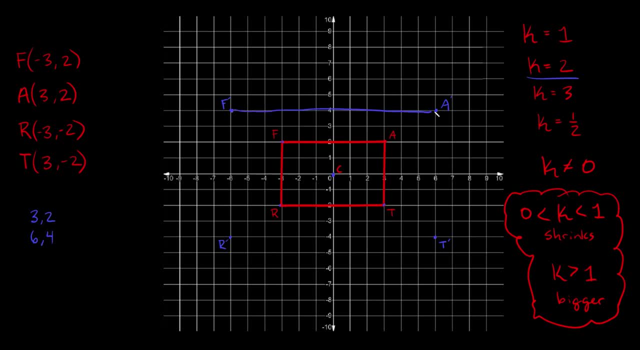 four corners of our rectangle, so we could just play, connect the dots. So now this copied rectangle, also known as the image, is twice as big as this original rectangle right, Also known as the pre-image. Now, that is the first method, just kind of counting squares. And now the second. 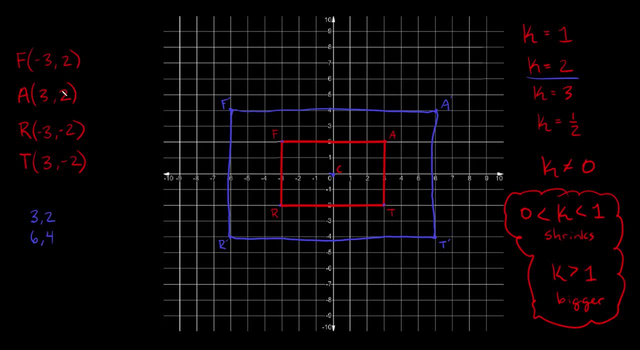 method, which is the pre-image, is the pre-image, which is the pre-image, which is the pre-image that we can use, is you can basically just list out the coordinates of your original shape right here. okay, So I have the coordinates right here. so F right now is at negative. 3, 2, right- Negative. 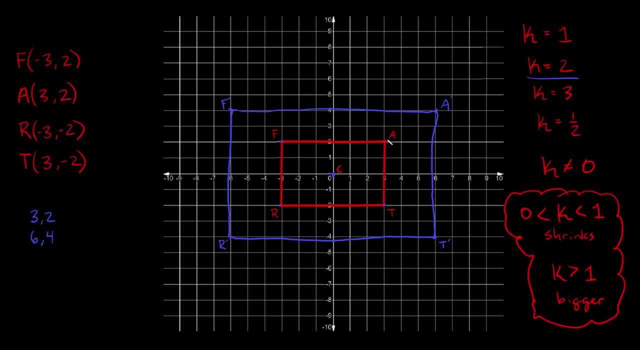 3, 2, F A is at 3, 2, right, 3, 2,. so. and then R and T are right there. okay, So all you have to do is take your scale factor. so remember, our scale factor over here was 2, right. So let's just write. 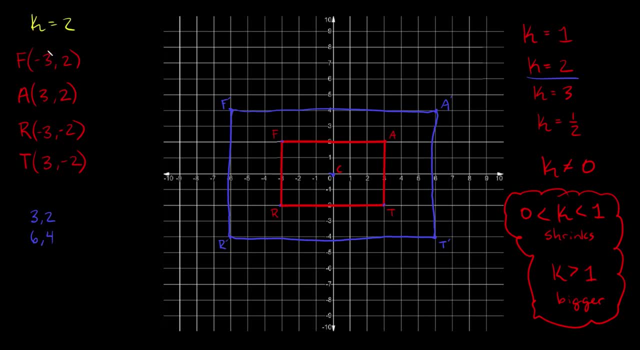 it over here. K is equal to 2, okay, So what you can do is just multiply all your coordinates over here by your scale factor, which is a 2, right? So we'd multiply this number by 2,, this number by 2,. 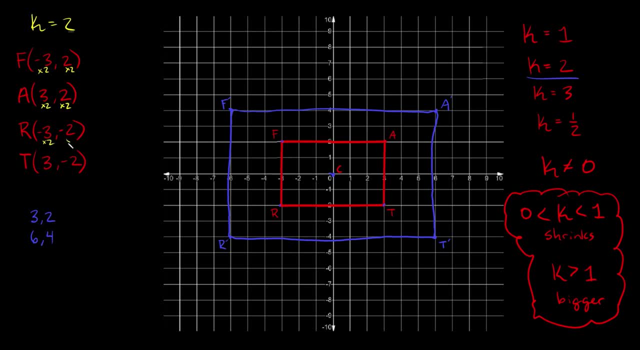 we'd multiply these by 2, multiply those by 2, and T. we'd multiply those by 2, right. So then here that means F prime would be at negative. 3 times 2 is equal to negative 6, right, And 2 times 2 is. 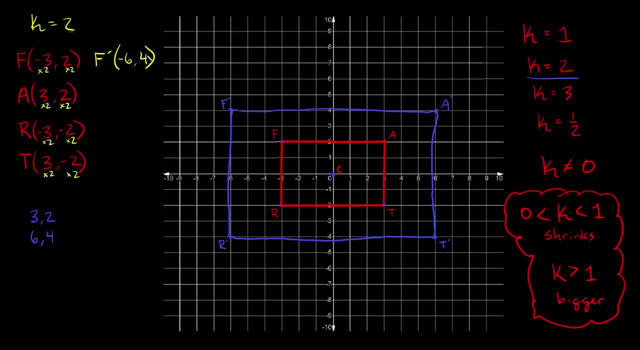 equal to 4, okay, So F prime should be at negative 6 comma 4.. So right now you can see that F prime over here is at negative 6, right, So F prime should be at negative 6 comma 4, right, So F prime. 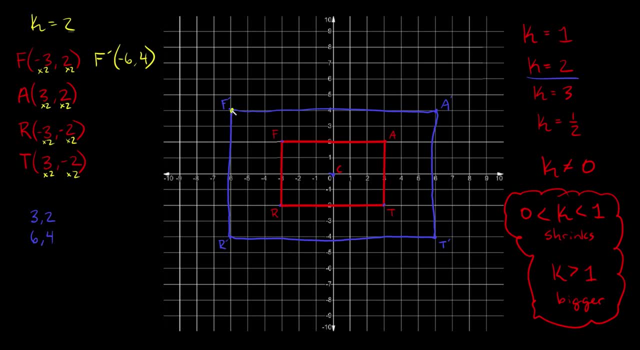 is in fact at negative 6, comma 4.. So then we land at that spot, right there. right? Same thing with A. So if we multiply these by 2, 3 times 2 is equal to. again, this is A prime. 3 times 2 is equal to. 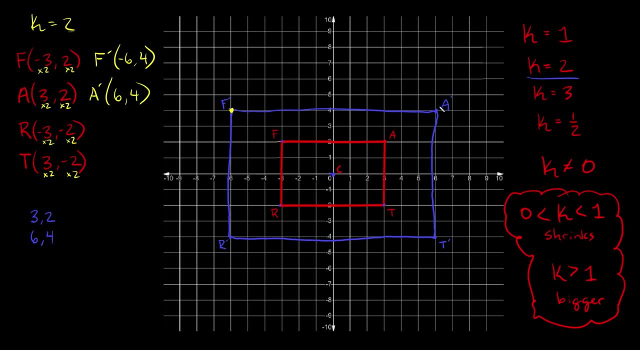 6, and 2 times 2 is equal to 4,, right. So then A prime should be at 6 comma 4,, 6 comma 4, and it is right. Same thing with R and T, okay. So multiplying all your coordinates by the scale factor is pretty. 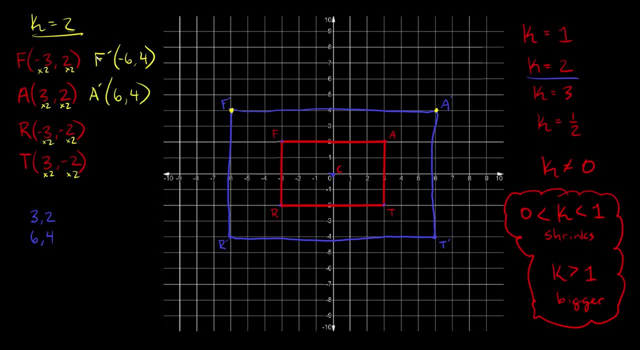 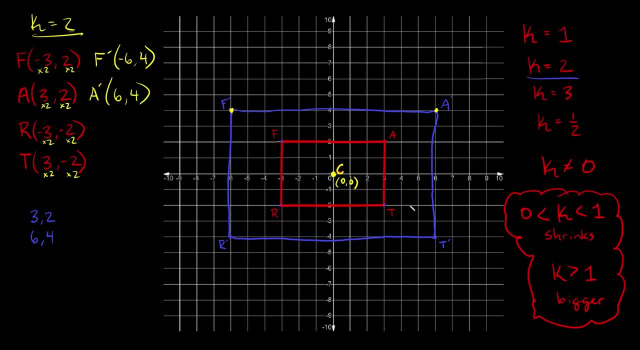 dilation is in fact at 0 comma 0, right. But if I moved this center of dilation anywhere else on the graph- right, If I moved it there, then this method no longer works and you'd have to use the first method of just counting the numbers. So if I moved this center of dilation anywhere else on the graph, 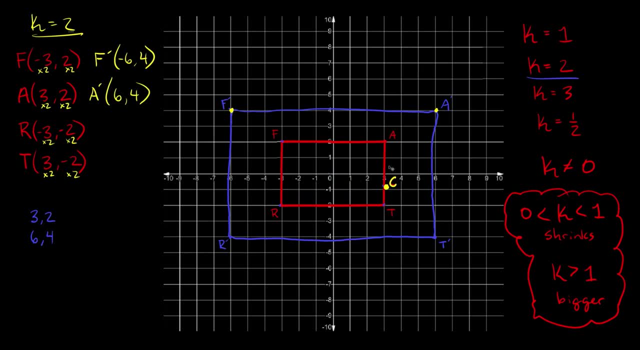 squares. okay. So if I moved this center of dilation anywhere else on the graph, you can't use this second method. okay, But if your center of dilation is right here at the center, at the very center, at the origin, then you can totally use this method okay. So let's try an example like that. 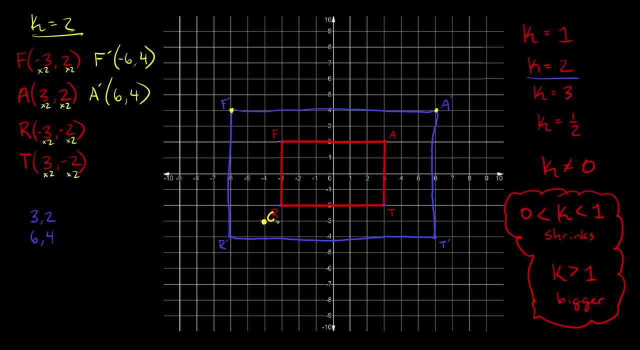 So let's take this center of dilation and we'll put it over here and we'll clean this up. So that's R, and now our center, or simply just dilation point, is right here. Okay, So now, if I want to, again, let's just apply the scale factor of 2, okay, So again I want to. 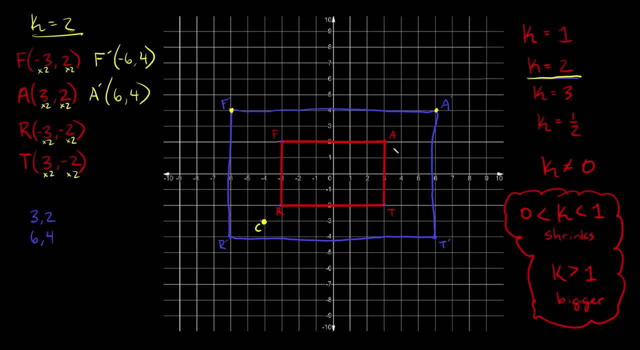 double this shape right, My original shape, the F-A-R-T in red. but now I have to start from this point out here, right? So again, just starting with F, What's the distance from C to F? How do? 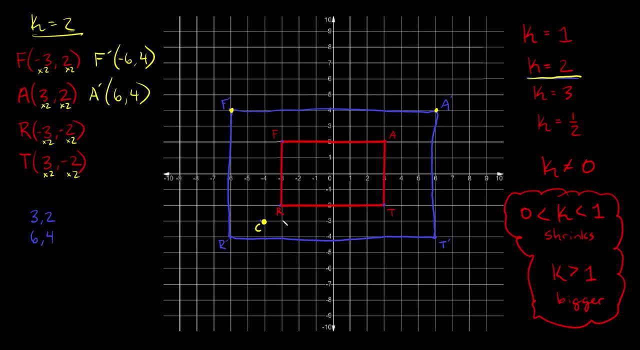 you get from C to F. Well, we can go over 1, and then we'd have to go up 3,, 4,, 5 spaces. okay, So we'd go over 1, and then up 5.. So that means we have to double that. 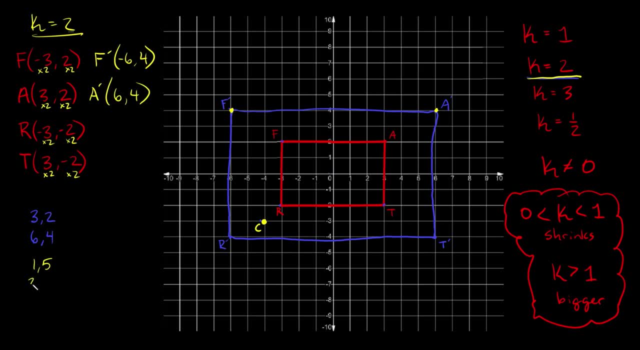 Right, So instead of going over 1 and up 5, we'd go over 2 and up 10, right, So we'd go over 2 and up 10.. So that's 3, and then 3 plus 7 is 10.. So 7's right there. Okay, so then this is now F. 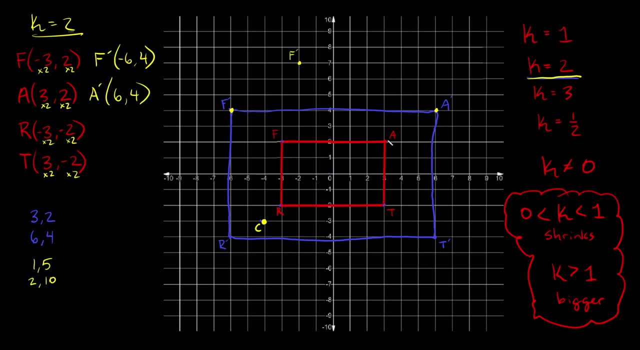 prime. okay, Now from C to A over here, how far is that? It's a lot farther. So from C to A, let's see, this is 4, 5,, 6,, 7.. So we're going to go right now. 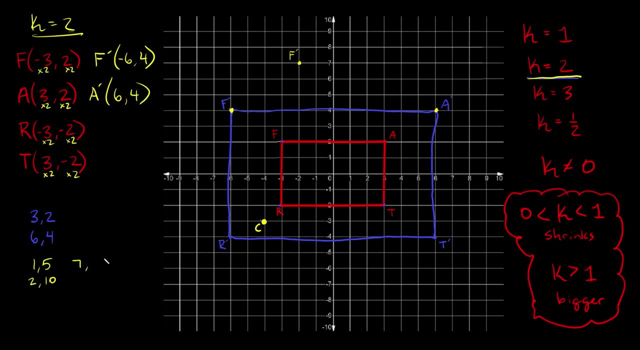 we just went over 7, and then we're going to go up 3,, 4,, 5.. Okay so if we want to double that again, we'd have to go over 14, and then up 10.. Okay so, here, go over 14.. So there's 4,. 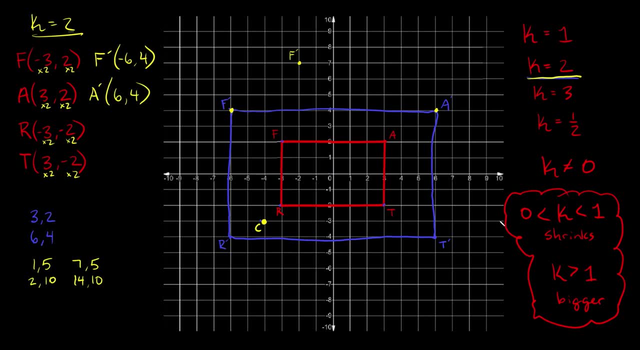 and then plus another 10.. It's actually right here. So that's 14 spaces, basically right there. and then up 10, right? So again up 3, and then plus another. 7 is 10, right there, Okay. 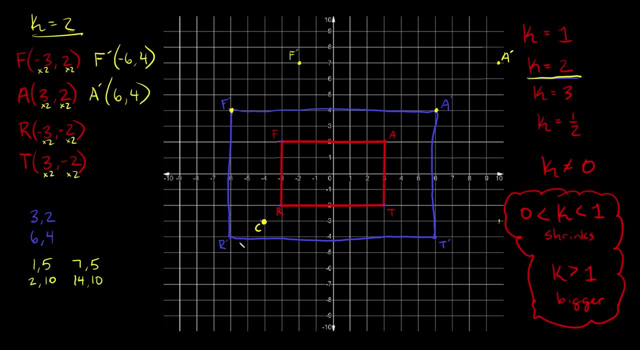 so then this point, right here is A prime, right Now, from C to R. well, it's one diagonal space. So if we double that we'd have two diagonal spaces right. So then R prime would be right there. Okay now, lastly, T, right, How far is it from C to T? 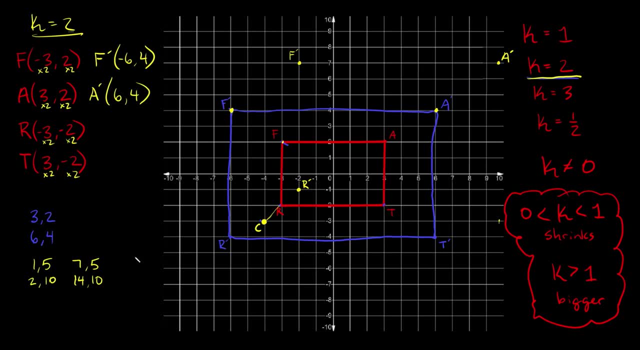 Well, right now it's 4,, 5,, 6,, 7, and then up 1.. So over 7,, up 1. So if we double, that be over 14, and then up 2, right. So then over 14, again would be right there, and then up 2. 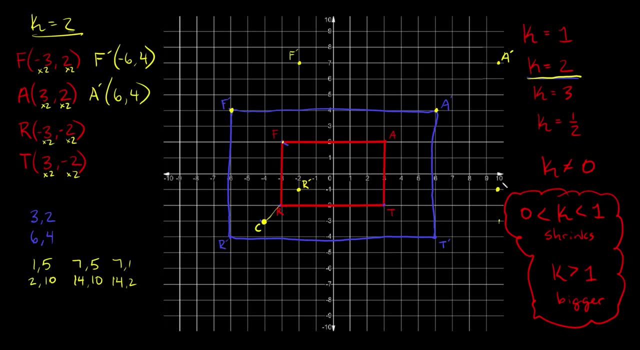 would be right there. So this spot, right there is T prime. Okay, So we have our four corners Right- F, A, R and T- So now we can play, connect the dots, There we go, Okay. so, as you can see, this triangle, the yellow triangle, is in a completely different position. 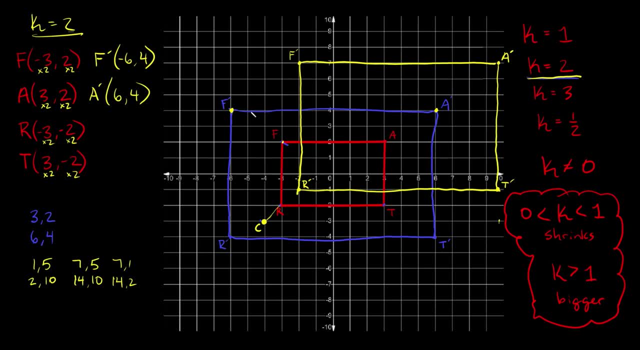 than the blue one, right, They're actually the exact same size—which makes sense, because they should both be exactly twice as big as the red one, which they are—but depending on your center of dilation, this thing is, it completely changes where you draw it. 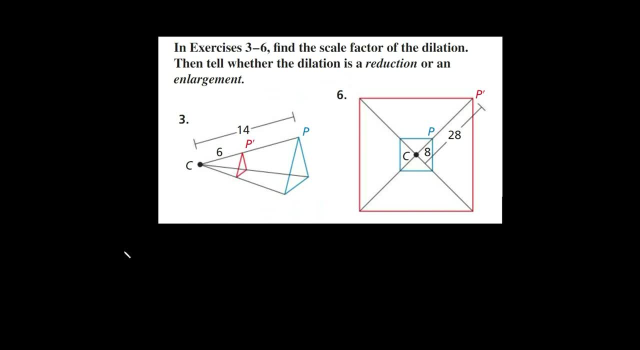 all, right now, the last thing I want to talk about is the scale factor. so sometimes you're not going to be given the scale factor. instead it's gonna be your job to find it okay. so here it says in exercises three through six: find the scale factor of the dilation, then tell whether the dilation is a reduction or 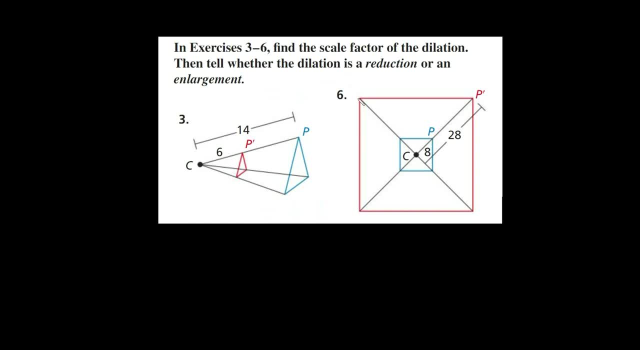 an enlargement, okay, so we're gonna do two of those examples, three and six, alright, so first of all, you can see, on number three, over here we have two shapes, right, so we have two triangles, a blue one and a red one. this one is labeled as P and this one is labeled as P prime. okay, so which one is the? 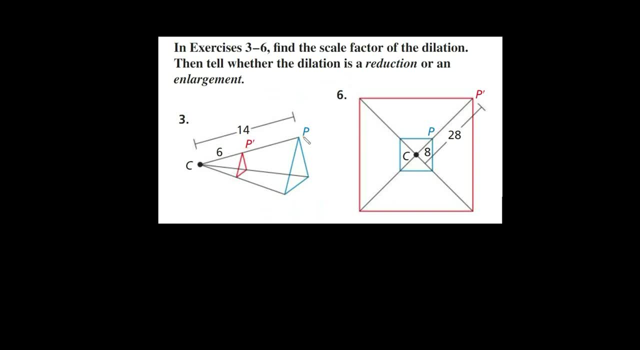 original and which one is the copy. well, P over here would be the original and P prime would be the copy right, and you can always tell, because the copies always have this prime symbol on them. okay, and it also gives us two lengths, so we have the distance. 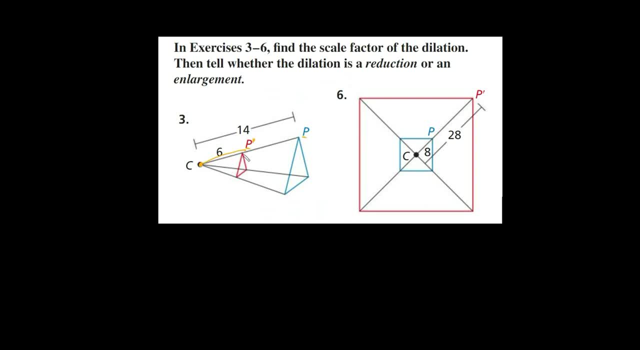 from the center of dilation to P prime, so that's six units, and we also have the distance from the center of dilation to P, which is 14 units, right? so if you're trying to figure out the scale factor over here, it's actually not too difficult. 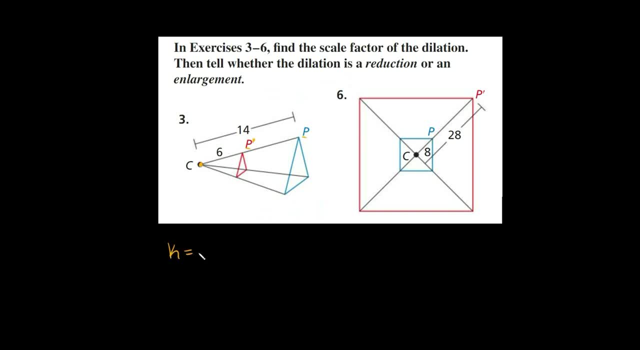 so all you need to remember is that the scale factor K is equal to the new length over or divided by the original length. okay, so just remember new over original, right? so in this case, what is the new length? well, that would be the distance from C to P prime, which would be equal to six. okay, and what was the original length? 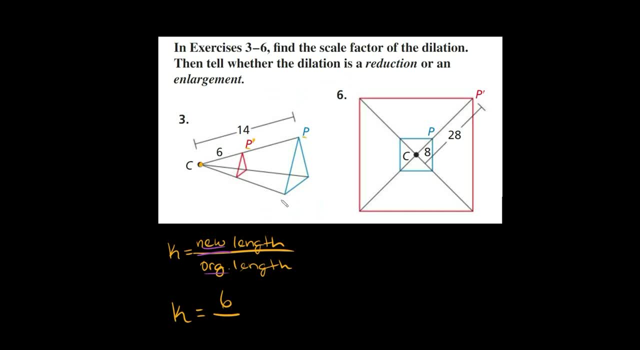 well, the distance from C to just P. right, the original shape is 14, right? so then your scale factor over here is equal to 6 over 14, and we can reduce that, right, we can reduce that down to three sevenths, okay, so here K is equal to three. 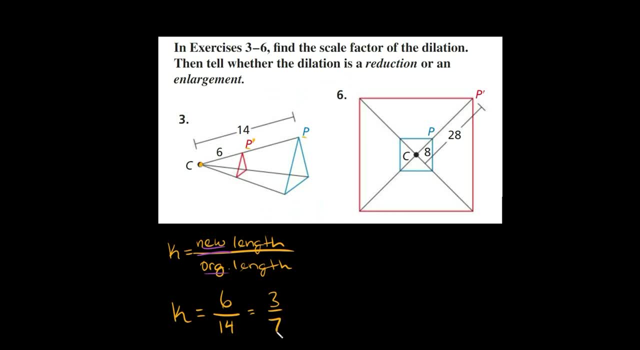 sevenths. okay, and is this a reduction or an enlargement? well, it would be a reduction, right? because this number 3, 7th, is between 0 and 1, and the other way you can tell is by just basically looking at the picture, right? so we have this. 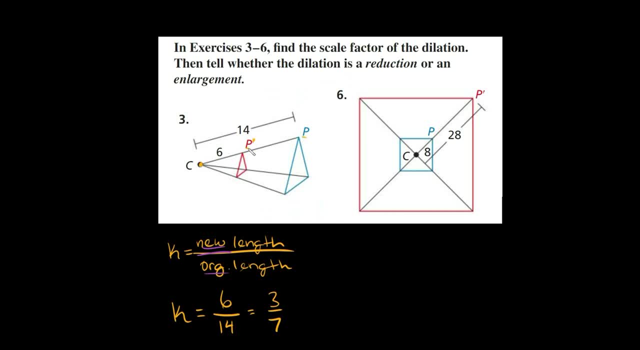 original shape, the big blue triangle, and then we reduced it down to 3, 7ths of its original size, down to this little red triangle. right there, alright, so not too bad, right? so let's just try one more. so again, we're trying to figure out what the 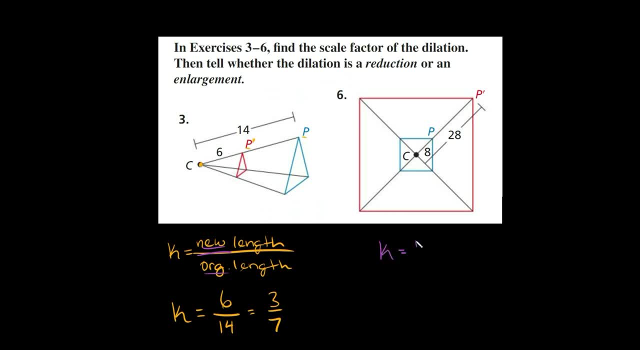 scale factor is right. so the scale factor again is the new length over the original length, right? so in this case, what is the new length? well, it again would be the distance from the center of dilation to your new spot. so that would be out over here, right? because p prime is in red, right? 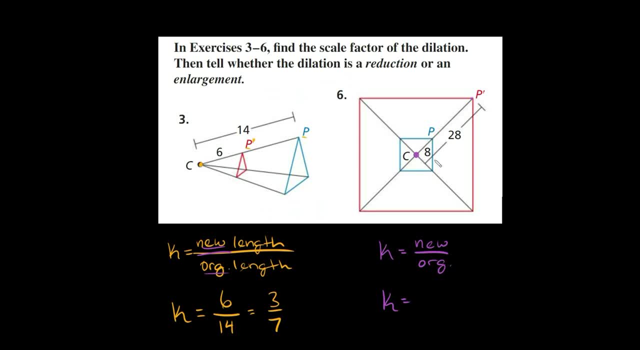 so that'd be the distance from c over here to p prime, and it looks like that distance is 28, right? so the new distance is 28, and then the original distance is right here from the center of dilation to p, which is right there. right, so this distance right here is 8, okay, and then we can. 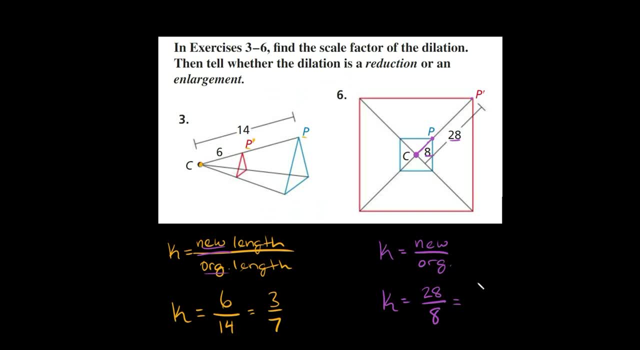 reduce this right. the top and bottom are both divisible by 4, so that reduces down to 7 over 2. okay, and we can rewrite this as three and a half, or we could write it as 3.5. okay, either way, same thing. these are just different ways that you're probably going to see these scale factors, but in either